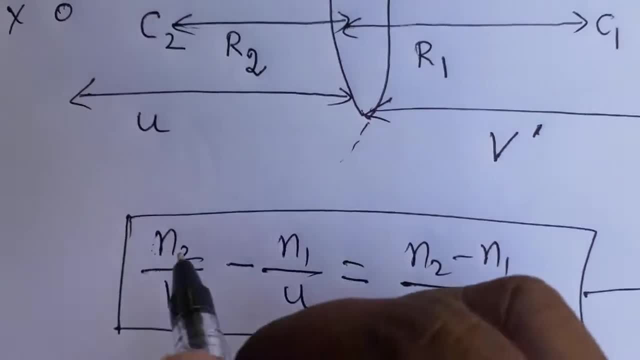 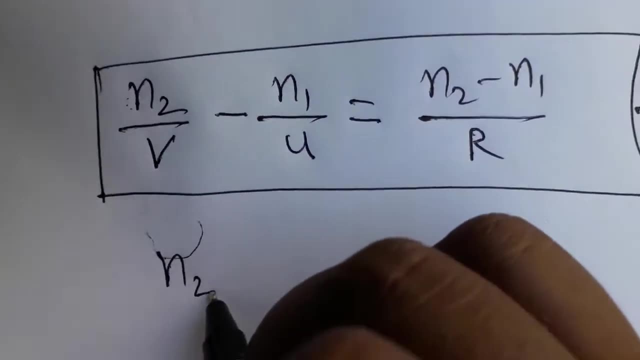 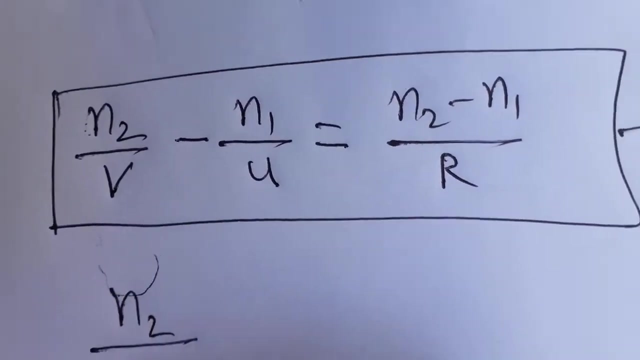 equation That I am going to use it. So here, first surface is refractive index of 1 and second, surface refractive index of 2.. So, as it is, equation will be N2, but here image distance will be. it is a image distance I am taken. as for first, surface is a V dash, So instead of write V, you can. 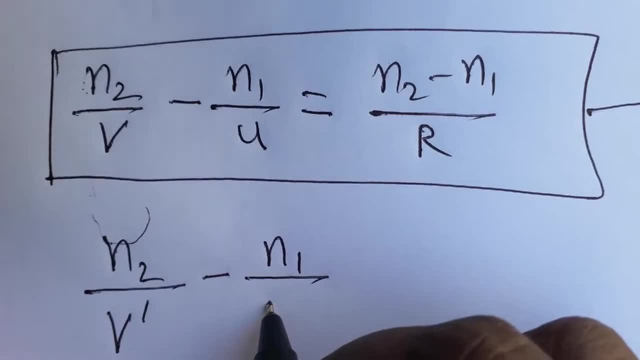 write as a V dash minus N1 divided by U is equal to N2.. So this is a V dash. So this is a V dash. This is a connection which is equal to N2 minus N1 divided by R one. So it is a ready. it happened. 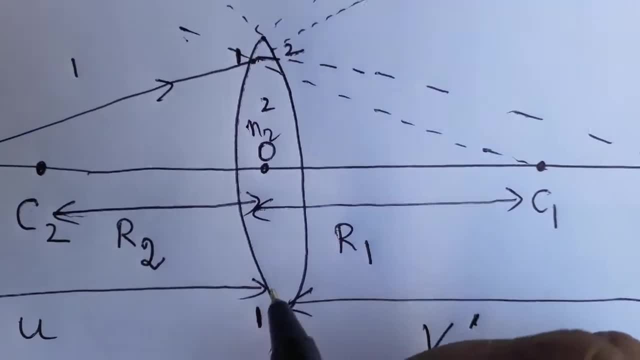 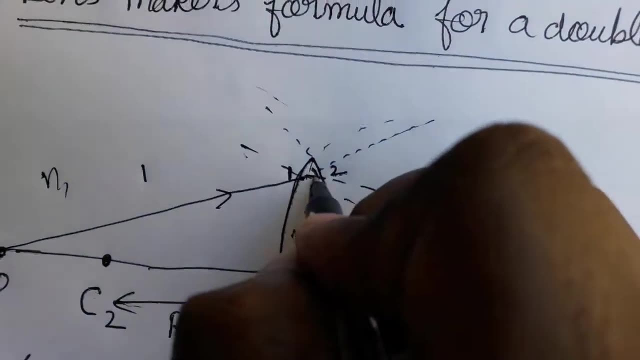 due to the radius of curvature. first to surface, to berthes of us to surface. this is a first to surface. now because of that I can't. it's going to deviate from it for key, So supply later. it maybe did it form here. No phone. here the object is going to shift. 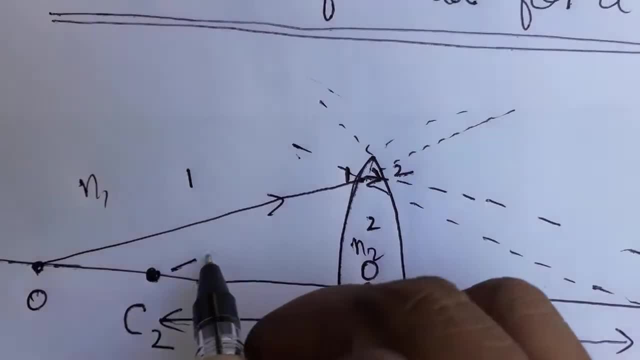 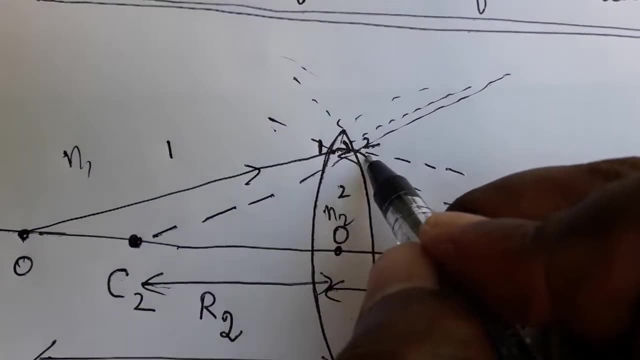 somewhere. The I am taken at the second surface, fasting curvature from here. So it is a normal for second surface. if its a light part, okay, it deviated away from the normal. the light is going to form like this. okay, the final image. 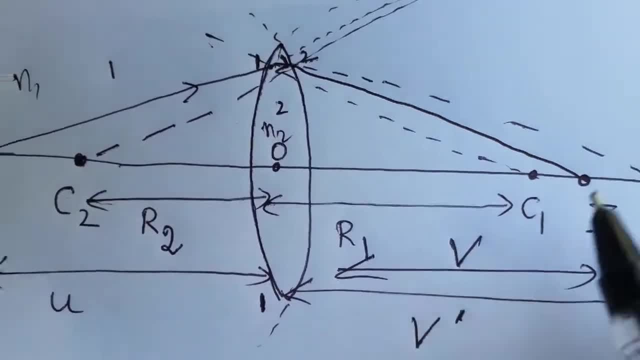 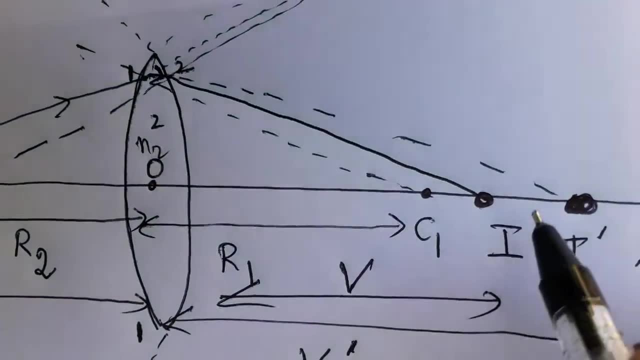 is formed at I at the distance of V. okay. so for O, object I dash is the image. okay. so when you are considering I dash is object, I is the image. okay. I will repeat again: O is object using a. 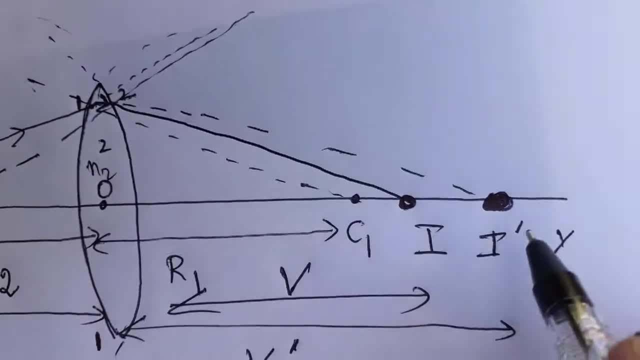 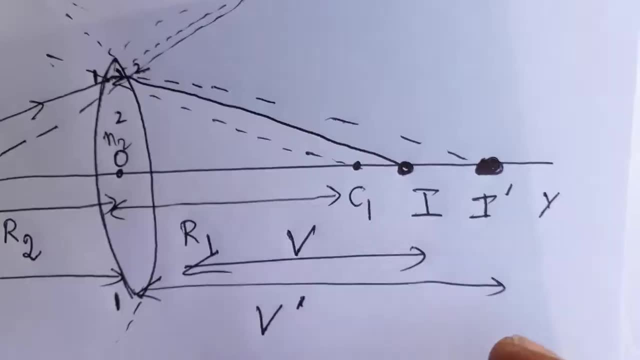 first surface, I dash is the image okay. when you are considering a second surface: okay, I dash is the object for final image okay. so I dash is the object for final image okay and V dash is the object distance. V is the image distance okay for final image. before we are taken. it is object. 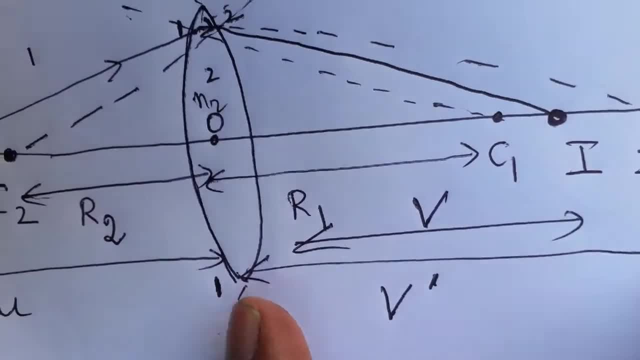 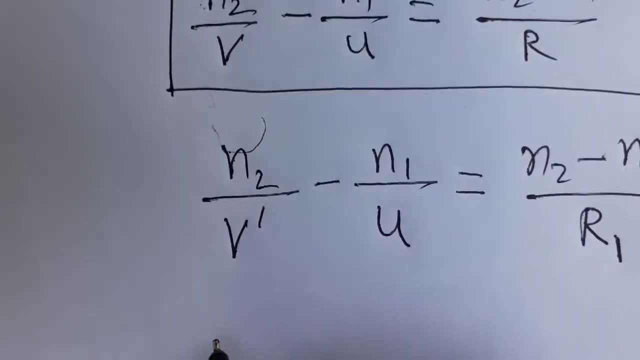 distance. V dash is the image distance. okay, now V dash is object distance, U is the image distance. and also light is traveling from second medium to first medium. okay, so this equation is going to change. it is according to the second surface to first surface, it is a first surface to second. 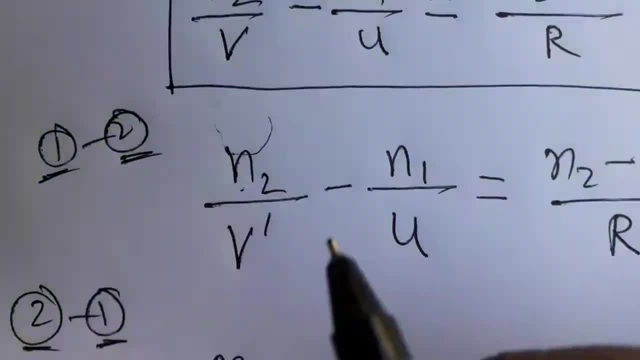 it is a first medium to second medium. it is second medium to first medium. okay, so the second medium to first medium. okay, so the second medium to first medium. okay, so the refractive index is going to be a first medium. object. it is a object distance, image distance. 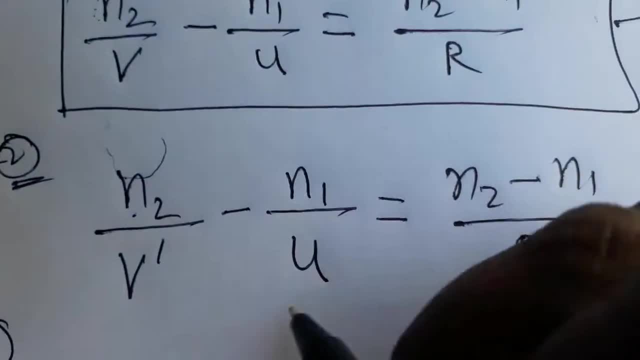 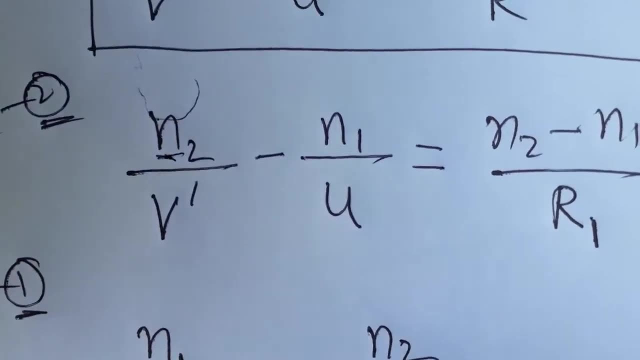 v dash is image distance. final image would form that v minus it is n 2. second medium is m 2. first medium is n 2. second medium is n 1.. So v is here u we are going to take it as a v dash, because now 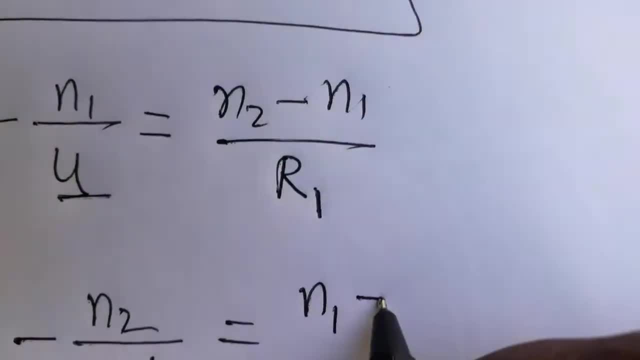 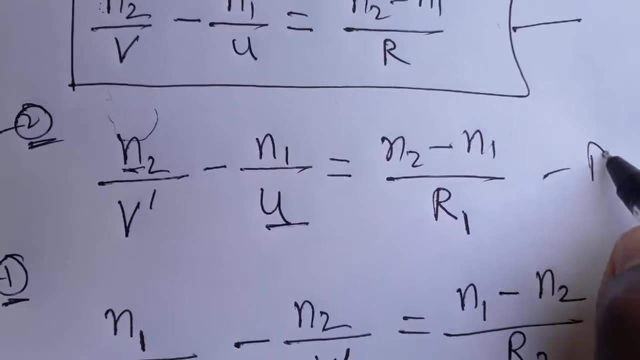 object: distance is v, dash n 2, we can take it n 1, n 1, we can take it n 2, but radius of curvature is r 2.. So just, I am adding both the equation, equation 1 and equation 2.. So when we are 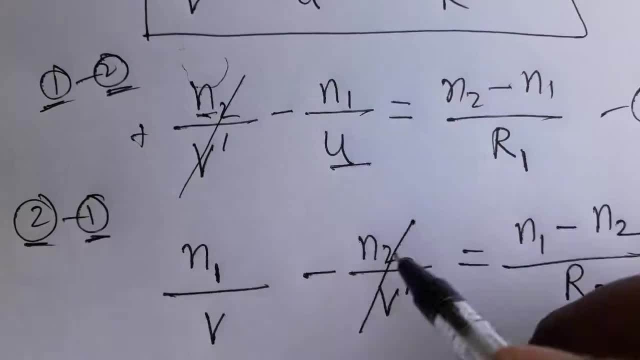 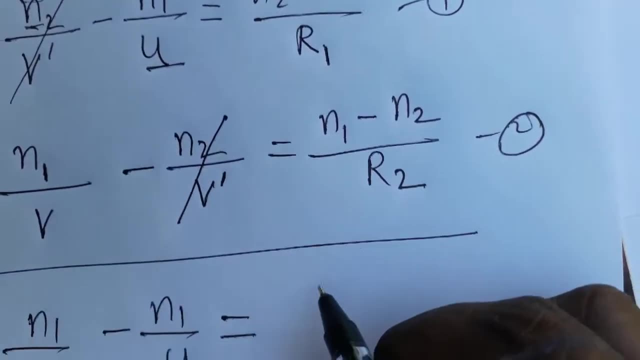 adding: it is a plus n 2 v dash minus n 2 v dash. just cancel this. 2 only will be there. n. 1 divided by v minus n 1 divided by u is equal to this one. it is n 2 minus n 1 divided by r 1 plus n 1 minus. 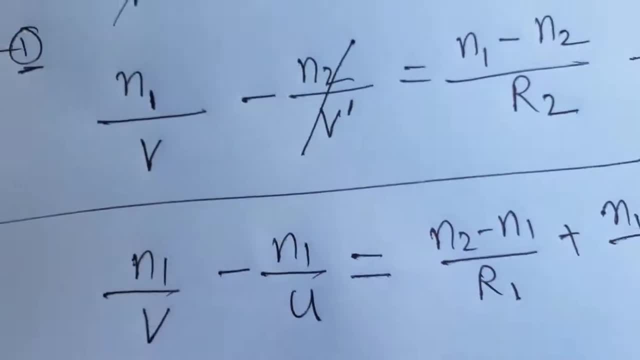 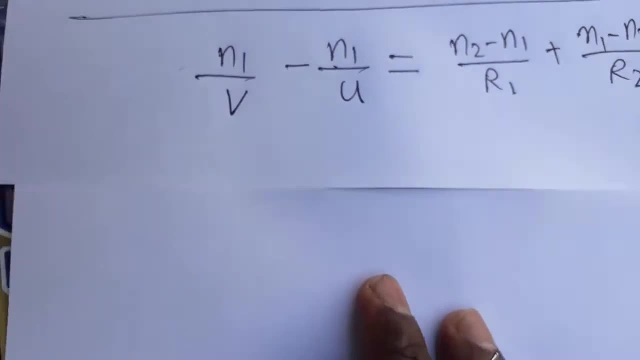 n. 2 divided by r 2. this equation we got finally, So I am taking this as a n in this equation, n as a common. From this equation I am taken n is a common, So that means what is going to happen. So 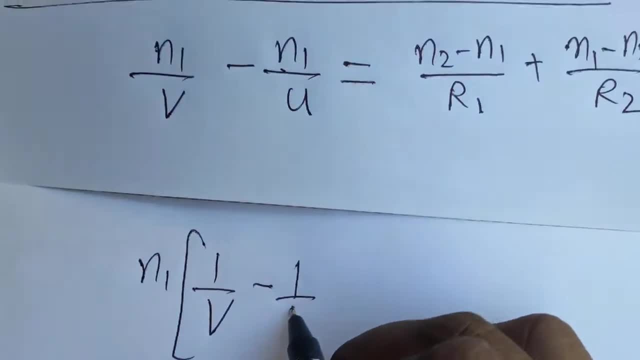 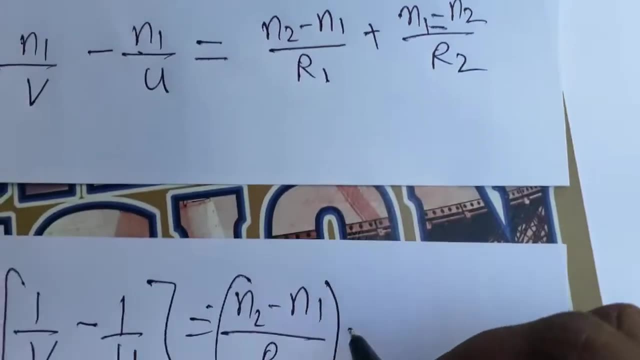 n 1, I am taken common 1 divided by v minus 1 divided by u, and here n 2 minus n 1 divided by r, 1, and this equation I am taken minus as a common. outside that means n 1, n 2 minus n 1 divided by r. 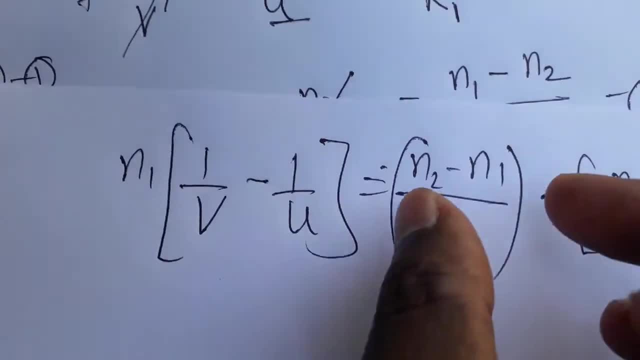 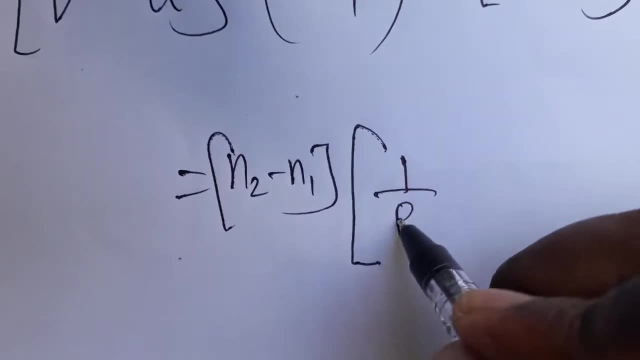 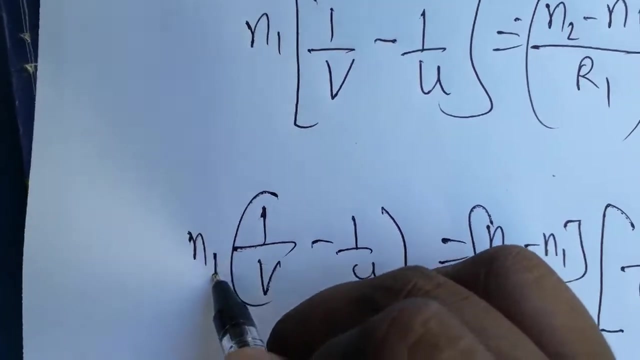 2.. Now we got like this equation. So here n 2 minus n 1, we can take it common for both the term so n 2 minus n 1.. So remaining So n 1 will be 1 by r 1 minus 1 divided by r 2. this side, 1 by v minus 1 by u, is a into n 1, n 1 from left side to right side. I am bringing cross multiplication. 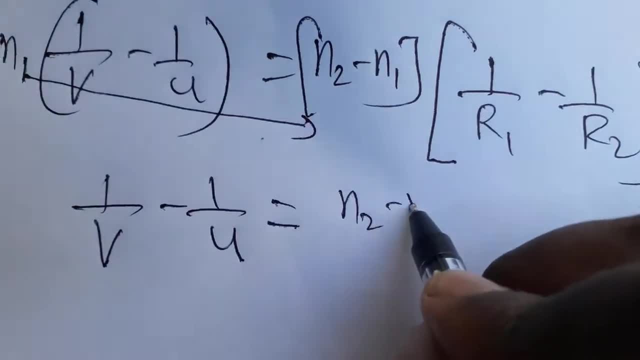 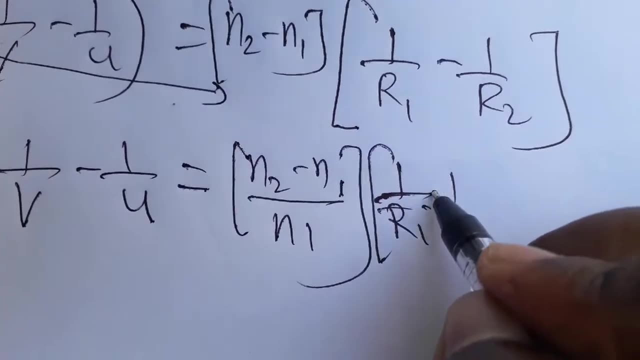 So 1 by v minus 1 by u is equal to n 2 minus n 1. divided by n 1 is equal to sorry into 1 divided by r 1 minus 1. divided by r 2, this equation will get: 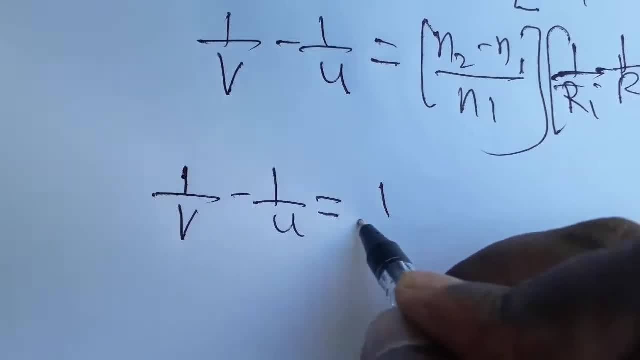 So 1 by v minus 1 by u is equal to 1 by n. 1. equal to 1 by f in lens maker, 1 by it is a formula for lens. it is a lens formula. 1 by v minus 1 by u.